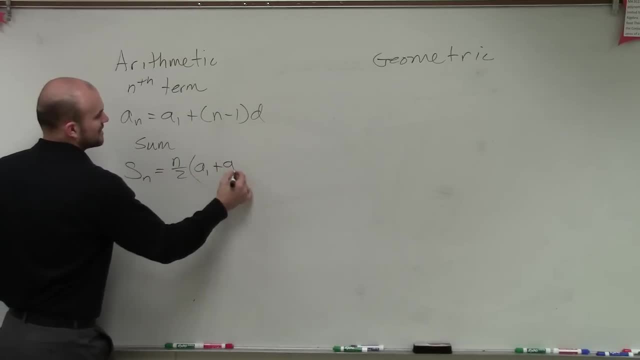 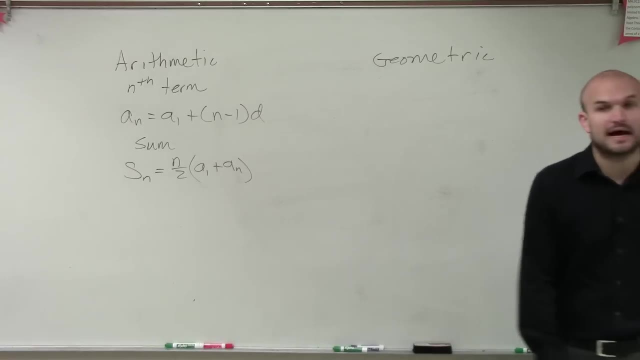 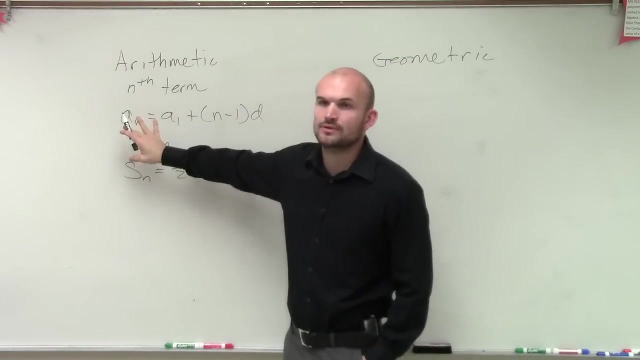 And divided by 2 times a sub 1 plus a sub n. Yes, Okay. So now what I'm going to do is introduce to you now the formulas for our geometric. Now one last thing, ladies and gentlemen, is just to remember when we did, when we were doing arithmetic with infinite, 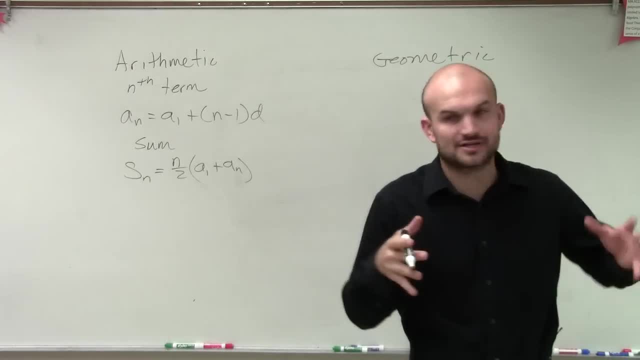 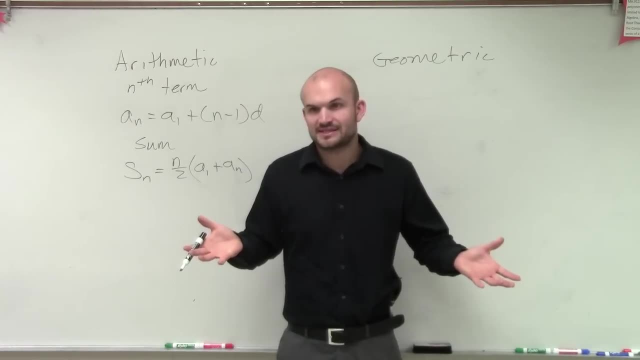 sums right. Remember when we kept on adding, like our fractions, they actually they went down to, you know, repeating, repeating decimals that we were able to convert to our fractions right To find the sum. So our sum kind of converged onto a fraction or a repeating decimal. that 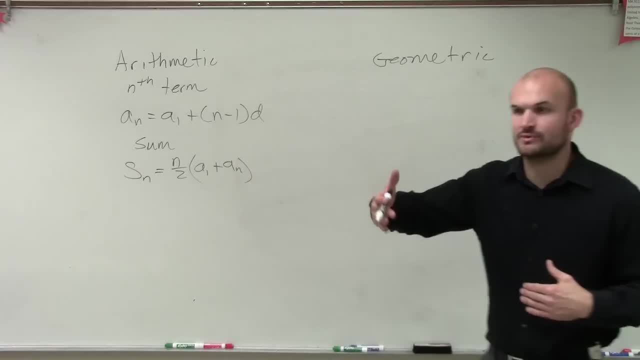 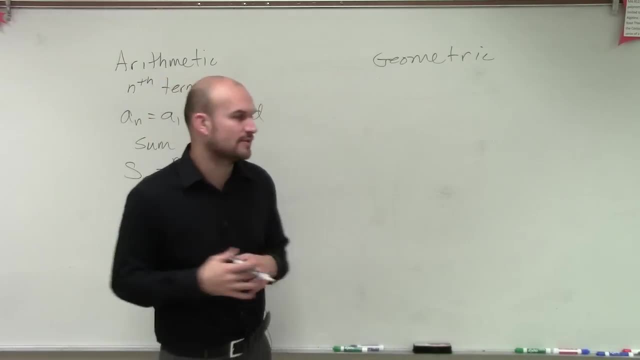 we used. all right, That's going to be a little bit different, though, with geometric, because all we were doing when we were finding an infinite sum is we just kept on adding, like a decimal point. We just kept on adding a decimal point, So it converged onto a fraction. 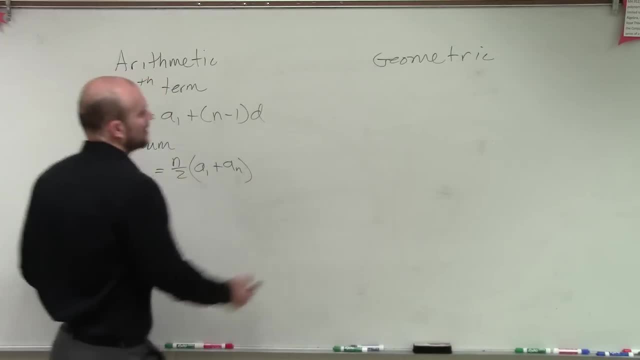 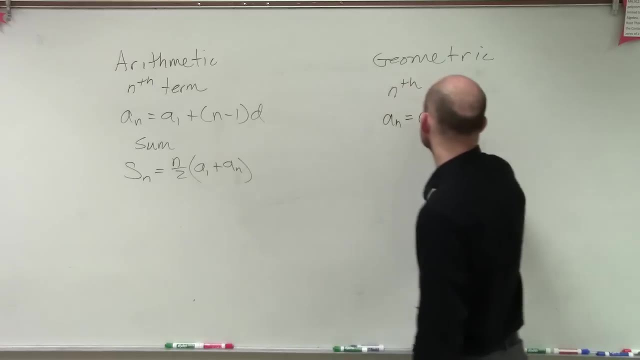 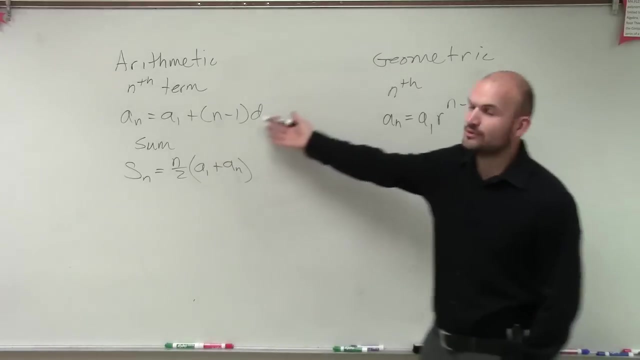 So geometric. all right, It's the exact same kind of parallels. We have a formula for the nth term. The formula for the nth term is: a of n equals a sub 1 times your original r times the n minus 1.. So now, in this case, if you remember, over here we had d, which 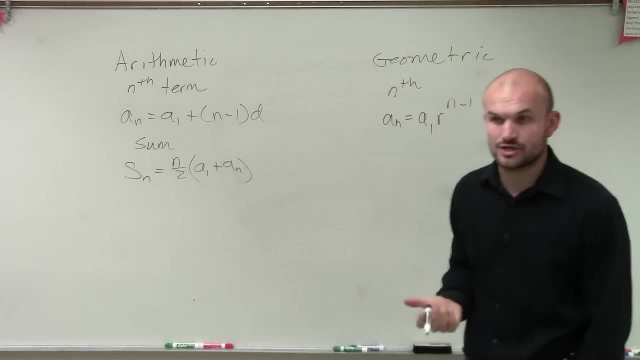 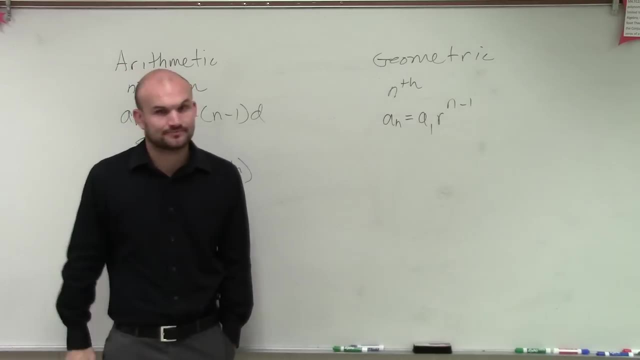 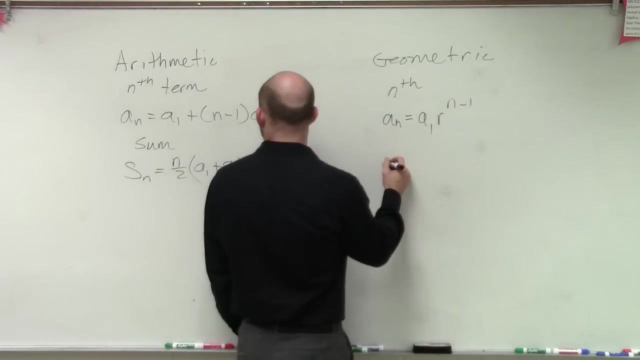 is our difference? Now we have r, which is going to determine our ratio, right, So it's: either we have to be given our ratio or now we're going to have to be able to define what the ratio is. all right, Got it Okay. Then we look at partial sum- all right, So let's. 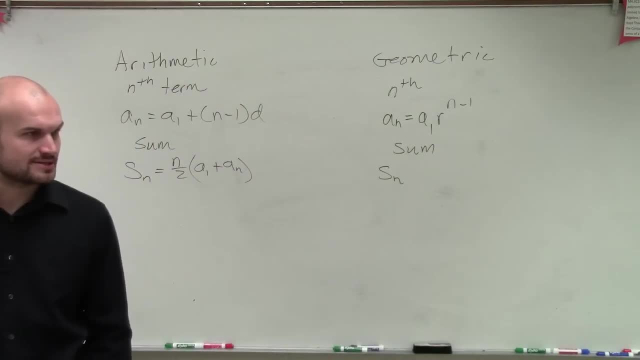 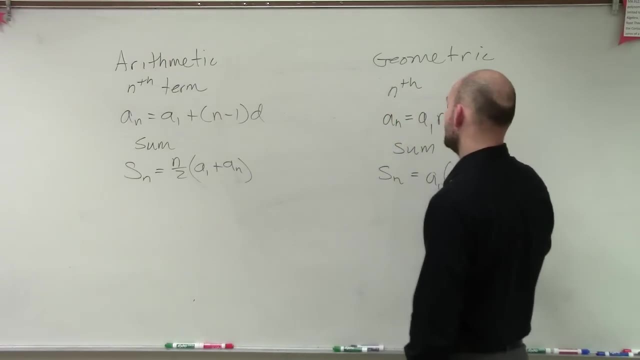 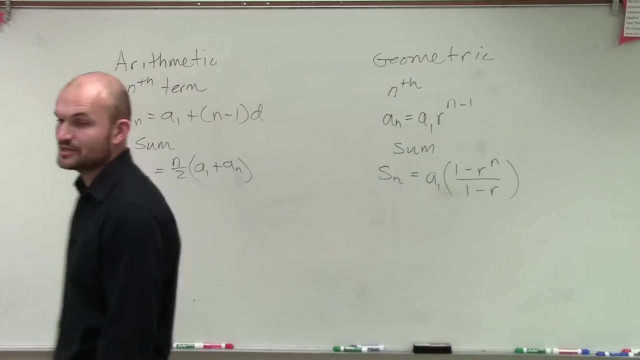 say, I want to say what is the partial sum of your geometric sequence? So we're going to have a little bit different formula here. We're going to have a sub 1 times 1 minus r to the n divided by 1 minus r. So again we're going to have to make 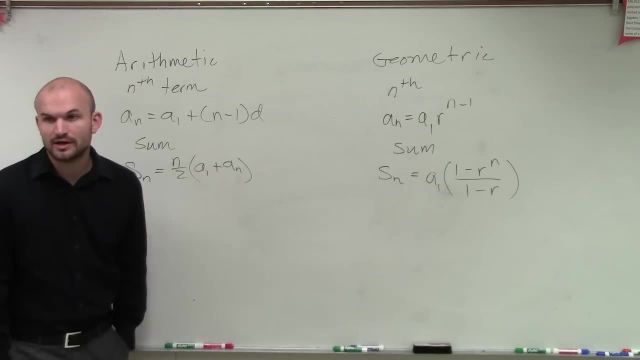 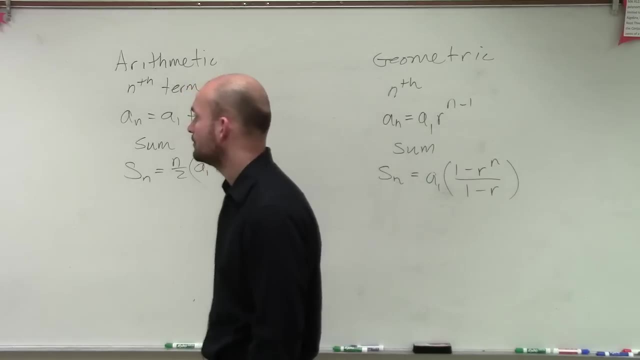 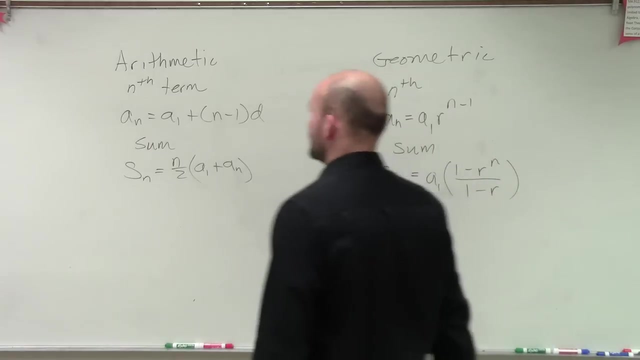 sure we know what r is. We're going to have to know our a sub 1 and our n A sub 1.. My little cheat sheet, My little cheat sheet. Are you serious? It's a sub 1.. I don't know why I wrote that over there.